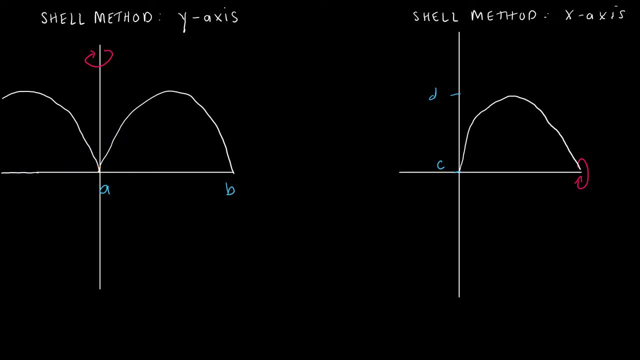 So what we're going to do now is do something called the shell method, and the shell method requires us to draw rectangles that are parallel to the axis of symmetry. So, again, if you can think about what each of these figures would look like, is I would have cylindrical shells or tubes. 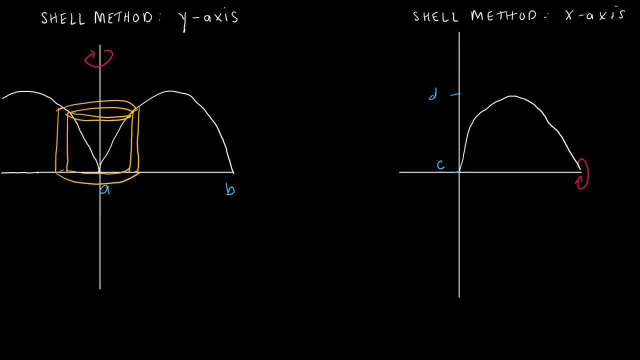 again many of them, and that's the difference here. Now I'm not going to take you through why the formula is the way it is. your book kind of takes you through that and it's pretty straightforward, but I'm just trying to make it not the longest video ever. 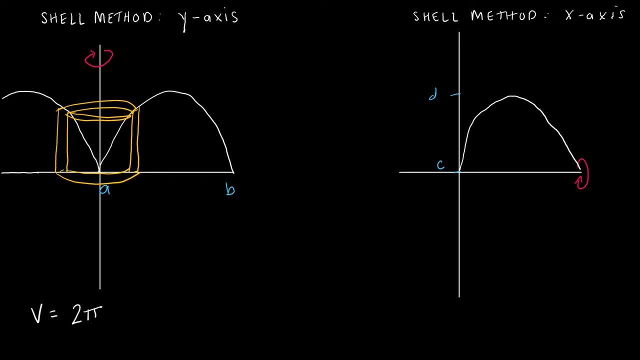 But that would explain why there's a 2 pi instead of just pi. So my formula here is 2 pi and then integrating from a to b, and then I'm going to take the radius with respect to x and then the height with respect to x. 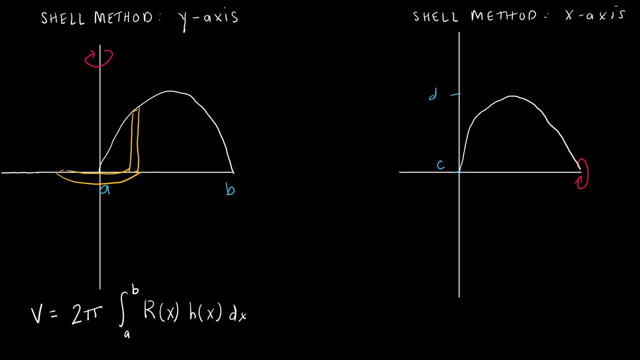 dx. So let's take a look at my figure so we can see which value is which. r of x would be the radius of the shape that's this guy. So again, if I had that figure on the other side, so from the y-axis to my representative rectangle would be the radius of my figure. 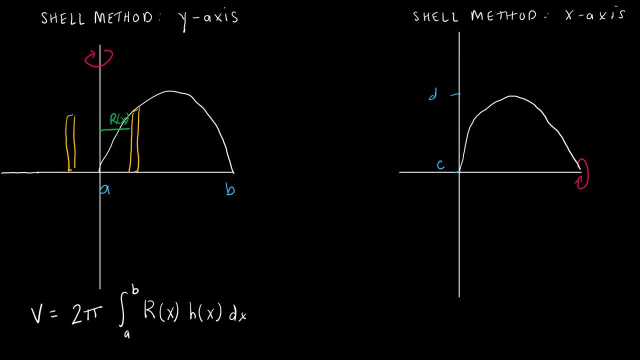 Then if I look at the h of x, h of x represents height, so this distance from here to here would of course be the height. So keep in mind that if I had, for instance, two figures that intersected, as I have in some of my other examples when I was doing area or volume, that h of x would be f of x. 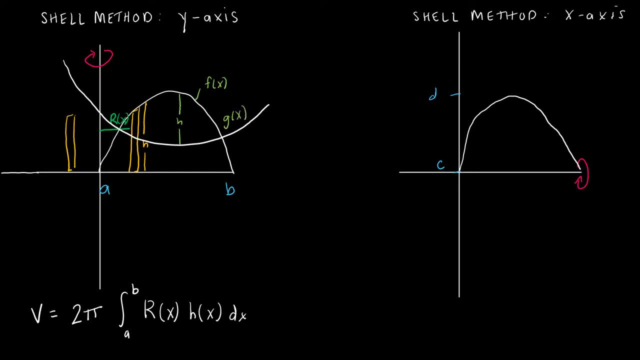 minus g of x Again, because we're trying to find the distance between the top of the curve and the bottom of the curve. So for my first example, h of x is just simply going to be h of x. Now, looking at the same method, but on the y, I'm sorry, the x-axis rotating about the x-axis- again what I'm looking. 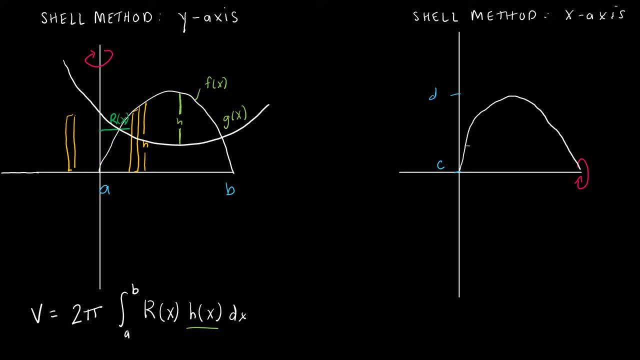 at is a rectangle that is parallel to the x-axis. So I'm looking at something like this Again. this would be reflected over and then my figure would be a shell or a tube that looks kind of like that. So if you can try to get a visual Again, looking at that formula, it's still 2 pi Now. 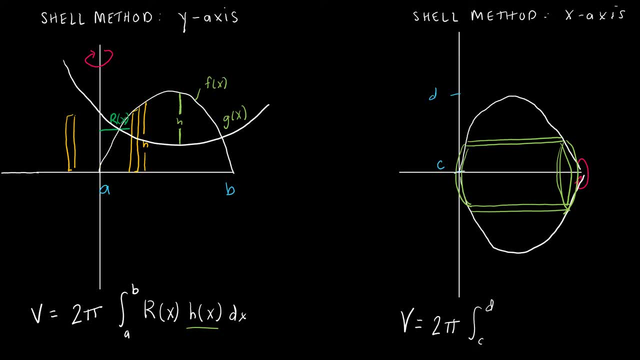 we're going to go from c to d just because quite often, when we're looking at integrating with respect to y, we use c and d instead of a and b, just for clarity. And we're still using the radius, but now it's the radius with respect to y. 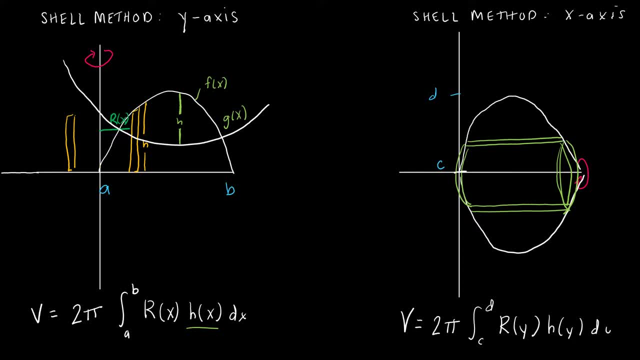 and the height with respect to y, dy And just as we talked about over here, it's possible that h of x is f of x minus g of x. So I'll write that down: f of x minus g of x. So over here that's really the same thing. The radius would be the distance from the x-axis. 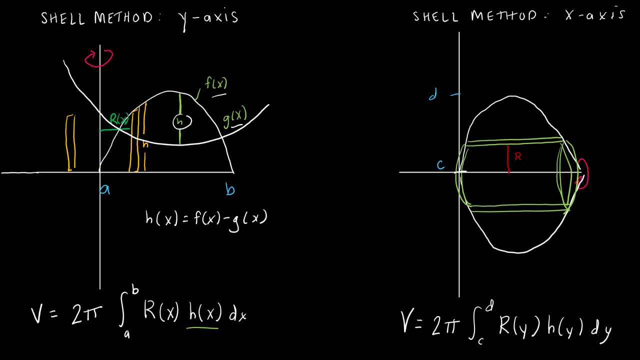 to my figure and the height is sort of like the width, so the height of the rectangle, again with respect to y. So this will make a lot more sense once we do some of these examples. but again, just to remind you, if you're. 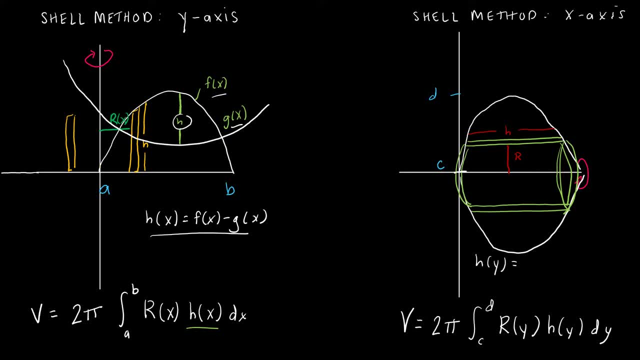 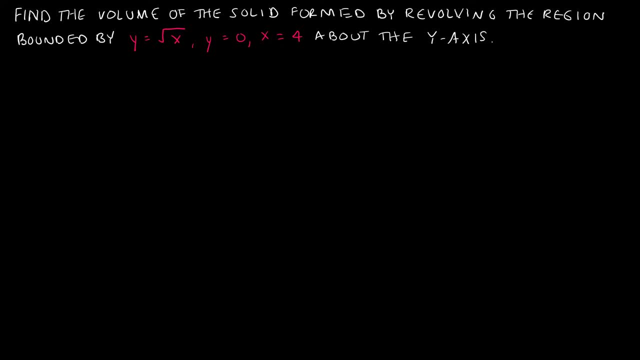 looking at the same thing. over here, we'll use the radius that's based on the height of the rectangle and the height of the rectangle, but just to make sure that you're having the same idea. So let's try and take a look at the first example together. I want to find the volume of the solid. 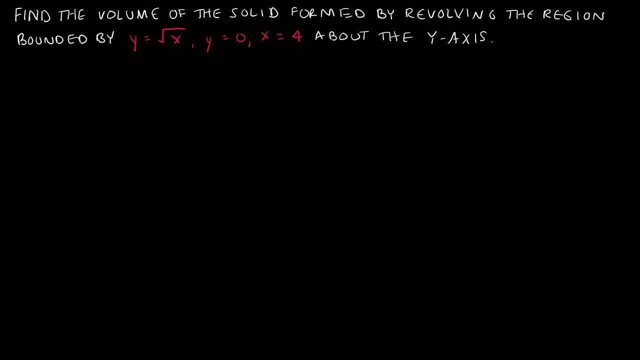 formed by revolving the region bounded by y equals radical x, y equals zero and x equals four. about the y-axis. So we're starting with a y-axis question so we can differentiate with respect to x. So, again, the first thing I would do is graph the volume of the solid. 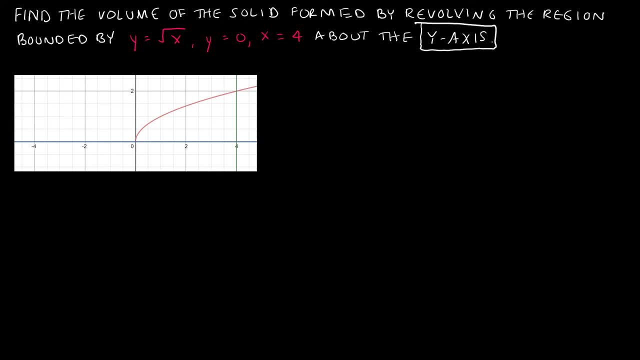 is graph. give me an idea of the figure that I'm working with- and, again, this is the region that we're talking about and rotating about the y-axis- would give me a reflection across the y-axis and keep in mind then that my representative rectangle would be parallel. 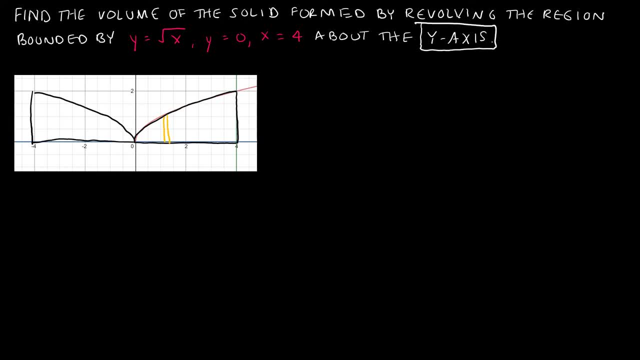 to the y-axis. So again, this distance is the radius and this distance is the height. So I'm going to copy down my formula, just so we remember. We have 2 pi again, from a to b, of r, of x h, of x, dx. 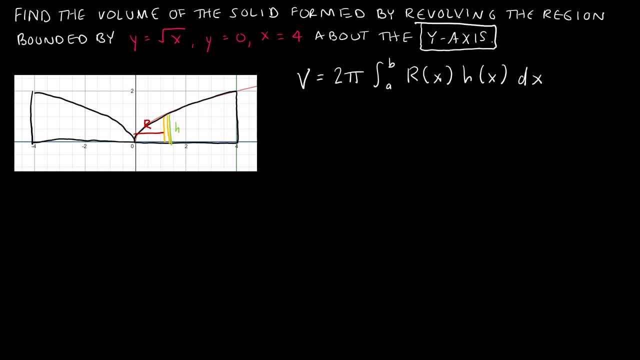 So what I need to do is think about how could I determine the distance of r, the radius, and how could I determine the distance of h or height? So, looking at the r value, I should keep with red, since I started with red. So, looking at radius, keep in mind that. 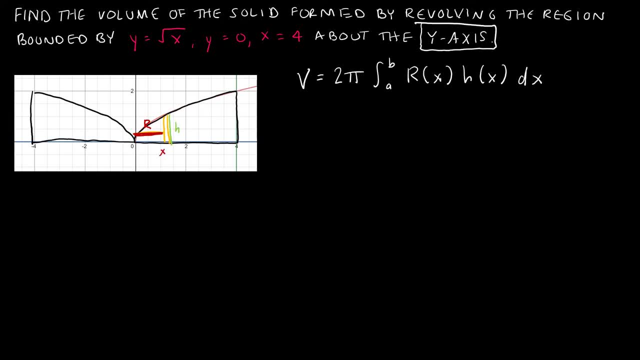 radius would be exactly what, whatever the x value is, That's how far the rectangle is from the y-axis- is the distance of x. That made it very easy that r of x is equal to x. Now what is the height of my rectangle? The height of my rectangle. 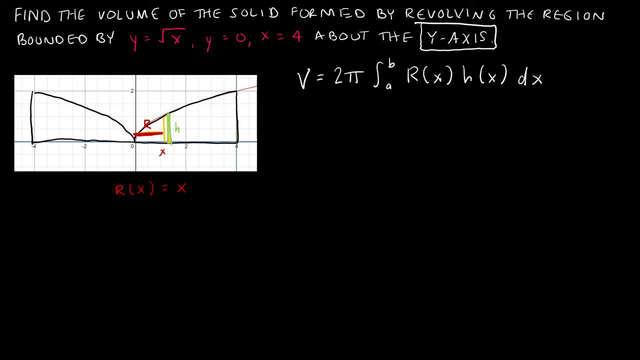 is just whatever my y value is. So if I think about this being my y value, of course, then my h of x is equal to y, but the problem is I can't use y because I'm differentiating- excuse me, integrating- with respect to x. So I need to think about what does that mean? Well, I know. 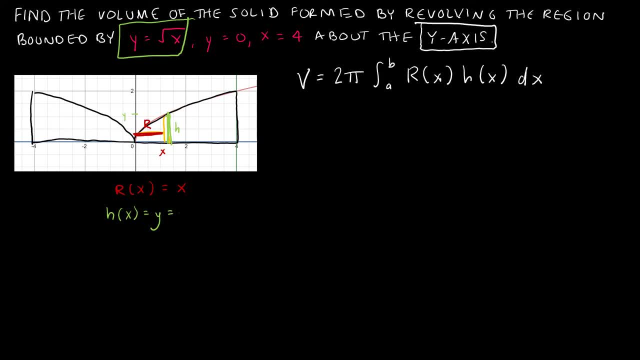 that the y value is going to be whatever the square root of x is based on this bound of my region. So that is how I'm going to solve this question, Again, with everything with respect to x. So let's start plugging values in. The volume is 2 pi From a to b, remember? I'm across. 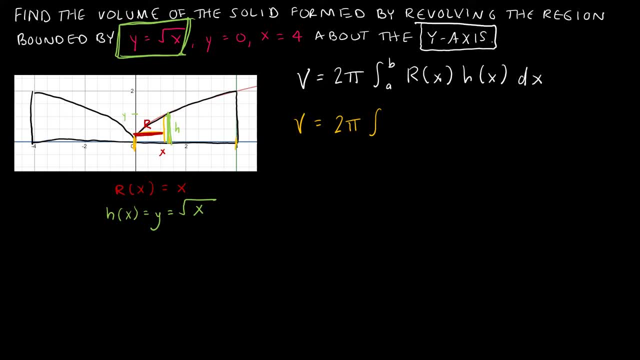 the y-axis, but I'm differentiating with respect to x, so it's from 1 to 4.. Again, that gives me, I'm sorry, from 0 to 4.. r of x is x, h of x. 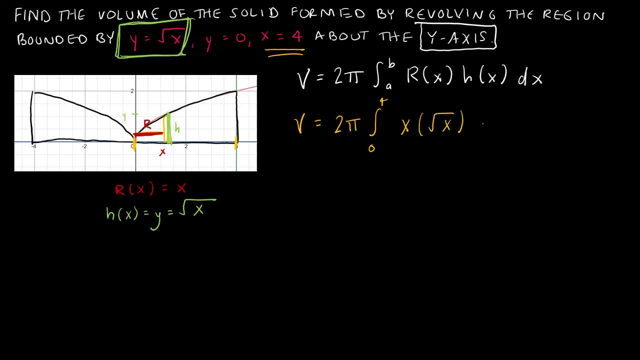 is radical x or root x. Doing some simplification, this is x to the first, This is x to the one-half, And so I have x to the three-halves, because our rule says: if we have the same base, we can add. 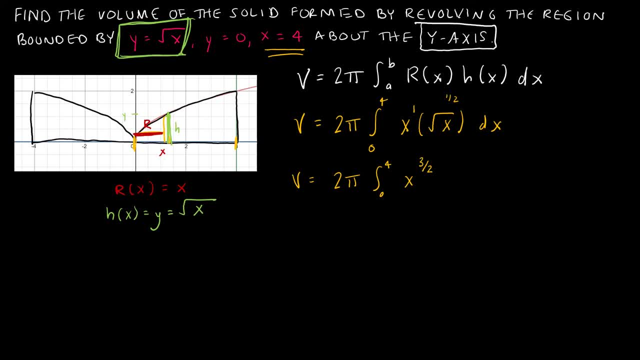 exponents. So x to the first and x to the one-half is x to the three-halves, because one is just two-halves. dx Again now I'm going to integrate. So the antiderivative of x to the three-halves is x to the. 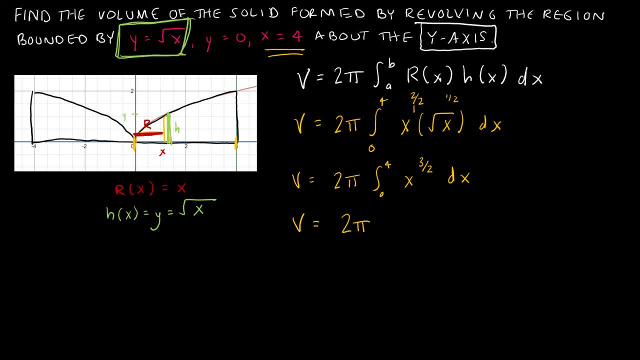 five-halves divided by five-halves. But of course I don't want to divide by five-halves. So I'm going to say this is x to the five-halves times two-fifths. So I'm just multiplying by the reciprocal. 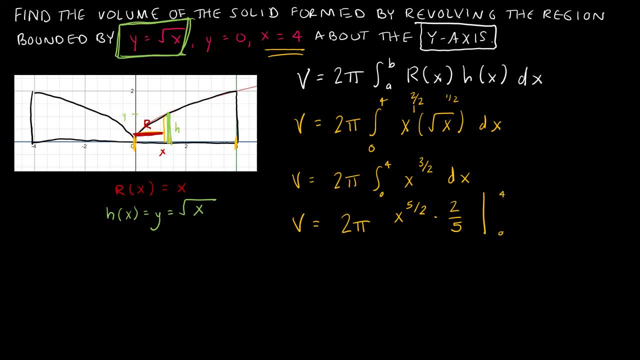 Again from 0 to 4.. So let's go ahead and work that out. I'm going to keep my 2 pi on the outside, and in fact I'm going to bring two-fifths to the outside as well, so that's going to give me 4 pi over 5 on the outside. 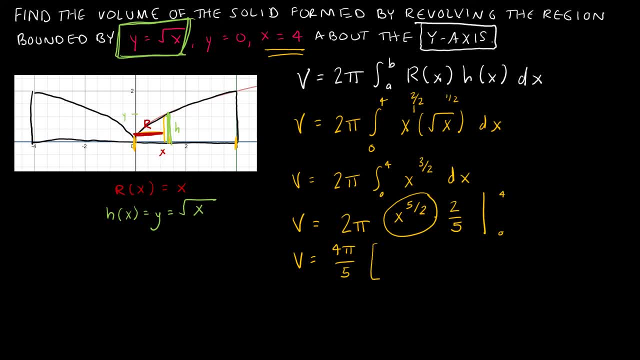 So I just have to deal with x to the five-halves for 4 and x to the five-halves for 0. So this is 4 to the five-halves minus 0 to the five-halves. I just added that and it will work, because x to the five-halves is just dropping x in that portion. 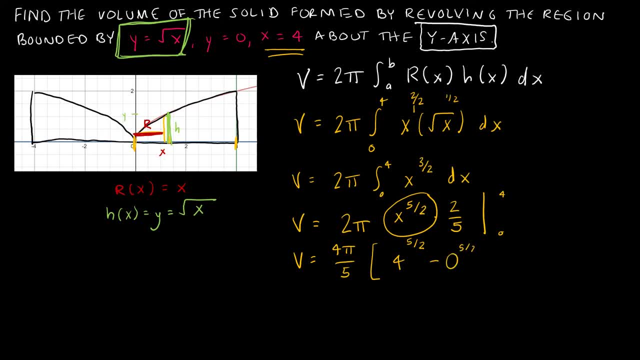 0 to the 5 halves. So I have 4 pi over 5, and then 4 to the 5 halves. Remember, this tells us to take the square root and this tells us to take that to the 5th power. So the square root of 4 is: 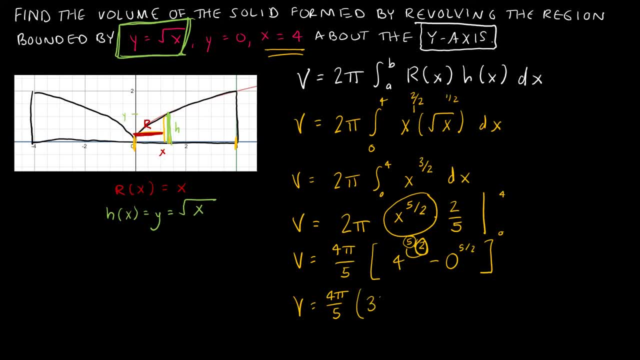 2.. 2 to the 5th power is 32.. And then, of course, 0 to the 5 halves is 0. So I have 4 pi over 5 times 32, and that gives me 128 pi over 5. for my final solution: 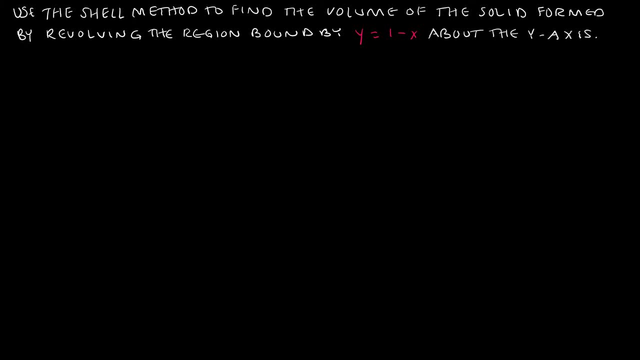 Here's another question for us to try, and this one's very similar to the last. So if you're feeling somewhat comfortable with it, go ahead and try this question on your own. When you're ready, press play to see how you did So. again, the first thing I would do 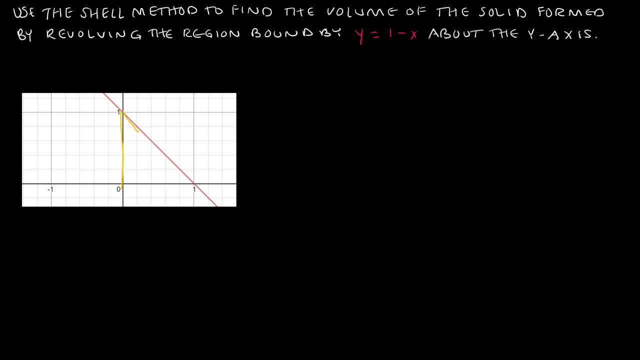 is, I'm going to take the square root of 4 to the 5th power and I'm going to take the square root is graph that function and I'm looking at a triangle. And again it didn't say explicitly: within the first quadrant, or also bound by x equals 0 and y equals 0, but that's what we're. 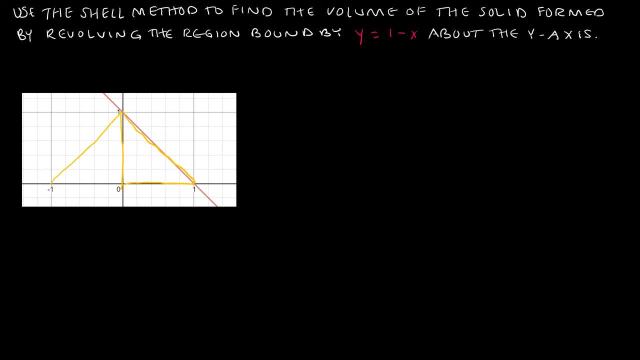 dealing with is this triangle, And if I revolve that around the y-axis, I would end up with this figure, And again we're thinking about a representative rectangle that is parallel to the y-axis, since we are revolving about the y-axis, So we're drawing that. 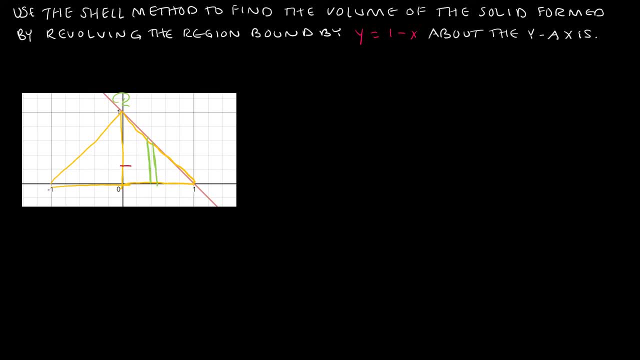 line parallel And, just as we did before, this region is r of x- Whoops, And I do want to point out that in your textbook it actually calls it p of x, but I think r makes more sense because it is a radius And again, this value is h of x. So, just as we did before, we need to think about. 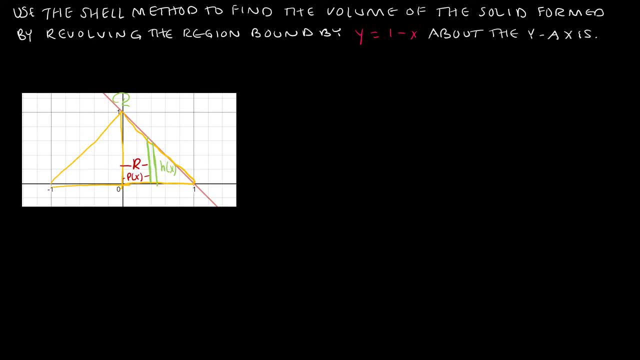 what represents r and what represents h. So if I'm looking at r of x, r of x, just like, my last example would be whatever the x value is, And h of x, just like on, my last example would be: 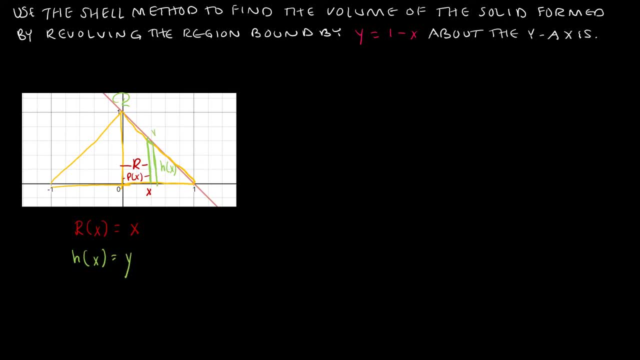 whatever the y value is. And again, I'm not able to put both x and y in my integral, so I'm replacing y with what function would give me the y value, which is 1 minus x. So now I'm going to. 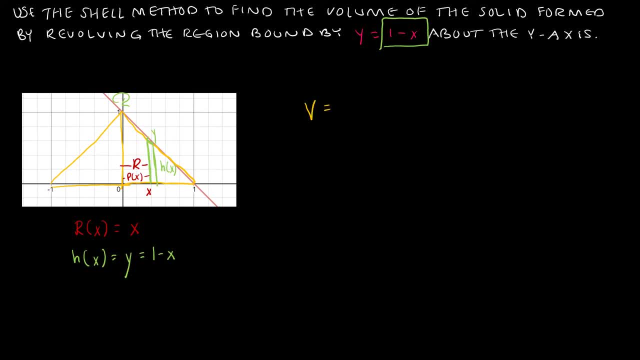 set up my integral. So to find the value of y, I'm going to set up my integral And I'm going to take 2 pi and then my limits are 0 and 1.. So from 0 to 1 of x for r of x and 1 minus x for h of x. 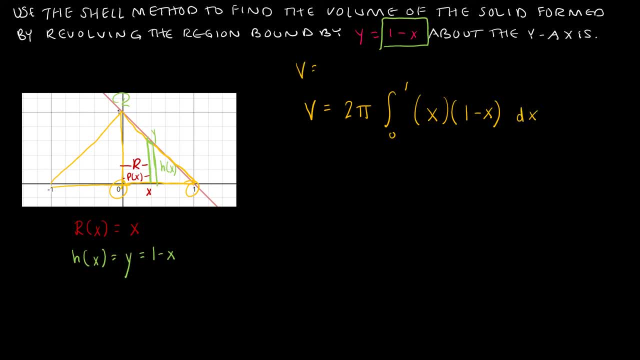 and then dx. So again, just to reiterate what the formula is: from a to b and then r of x, h of x and then dx. So again, keep in mind that this could also be called p of x, if you're looking at. 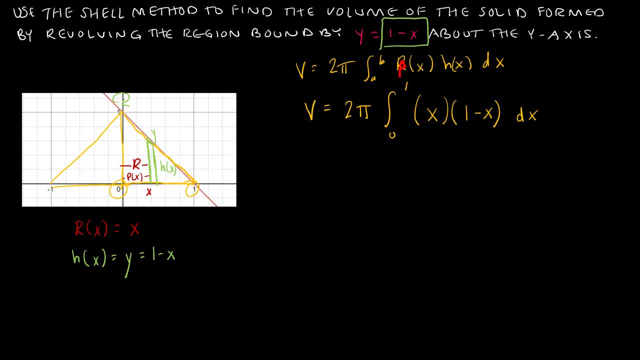 your textbook. So pretty easy integration on this one. I have 2 pi and then this is from 0 to 1, and I'm going to distribute the x, So I have x minus x squared dx To integrate. 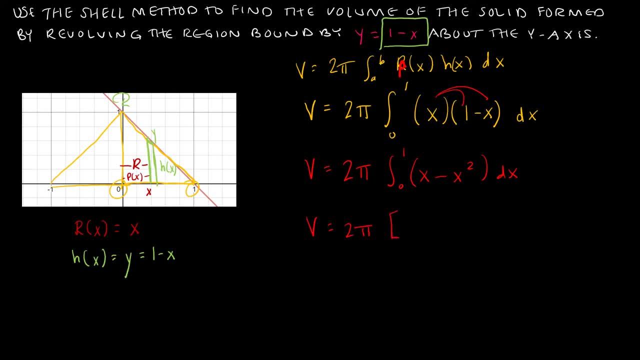 I have again using the power rule. I'm increasing the exponent by 1 and dividing by that exponent, So x squared over 2, and then x cubed over 3, and evaluating from 0 to 1.. So I have 2 pi. Plugging in 1, I get 1 half minus 1 third. 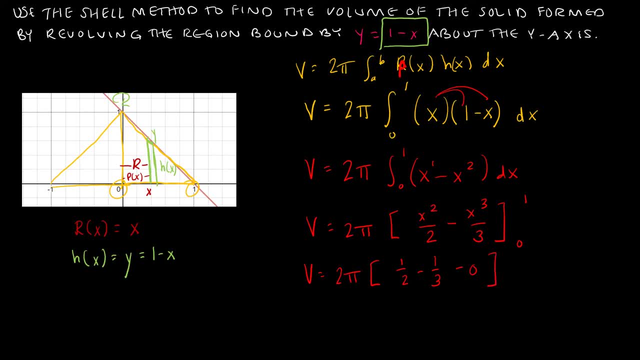 Plugging in 0, I would get 0.. Again, you can combine these by making a common denominator. So multiplying that first fraction by top and bottom by 3, gives me 3 sixths. Multiplying the second fraction, top and bottom, by 2, gives me 2 sixths. 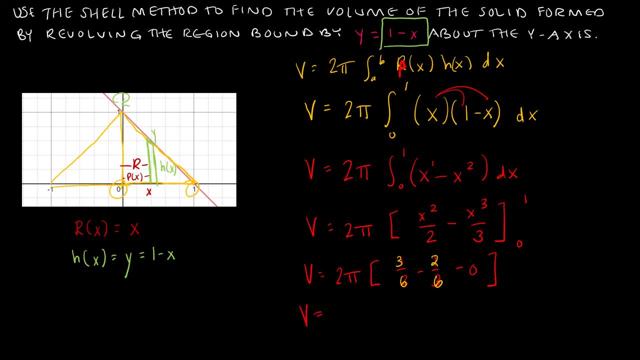 So I have: the volume is equal to 2 pi times 3 sixths. minus 2 sixths is 1 sixths. So that gives me 2 pi over 6, which reduces to pi over 3.. So that is, my volume is pi over 3.. 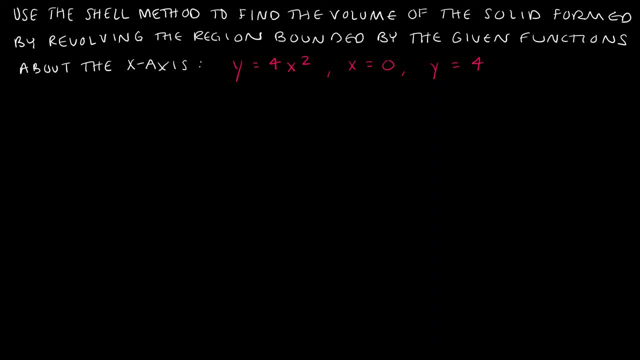 Let's take a look now at an example where we are revolving our function or our region about the x-axis. So obviously that means we are going to differentiate or integrate- excuse me- with respect to y. So again, the first thing I would do is to: 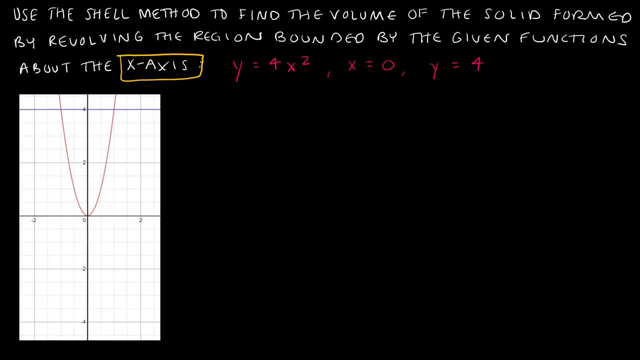 graph the function, And I'm using Desmos, as I always do, just to make it easier- And I'm looking at the region bound by: x equals 0,, y equals 4, and that function. So I'm looking just at the right. 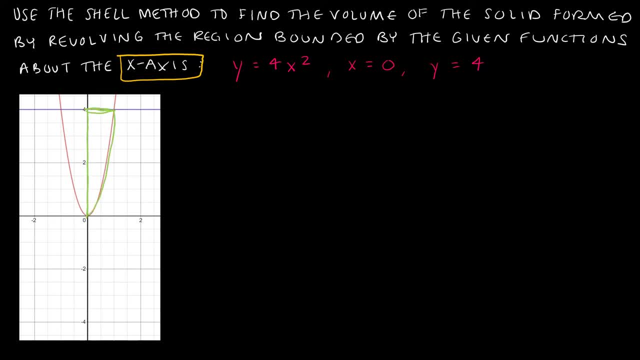 side of this parabola right here, And then again that would be revolved or reflected across, and it is actually being revolved around. So, again, thinking about that representative rectangle would be parallel to the x-axis, And again, 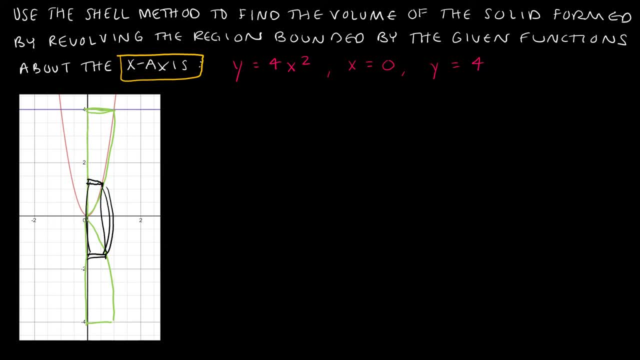 we're thinking about the shells that would look like this- I know my artistic ability is astounding. So, again, we need to think now about our formula. And our formula for volume is 2 pi, and then c to d and then r of y, or your book calls that p of y, h of y, dy. So that's our function. 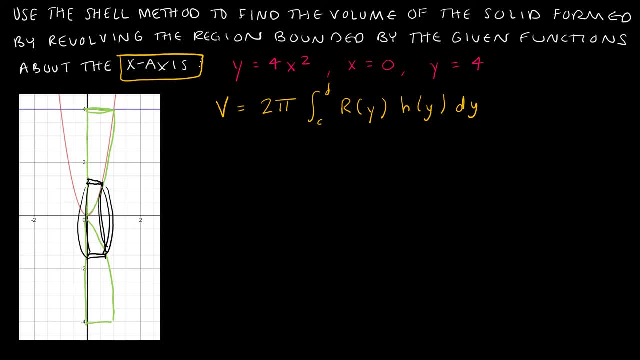 And so now we just have to determine what each of those values are. So I'm going to clean up my cute picture And again think just about this rectangle. And the radius would be the distance from our axis of revolution, which is our x-axis, to our function. So that's r of y, And then our height would be. 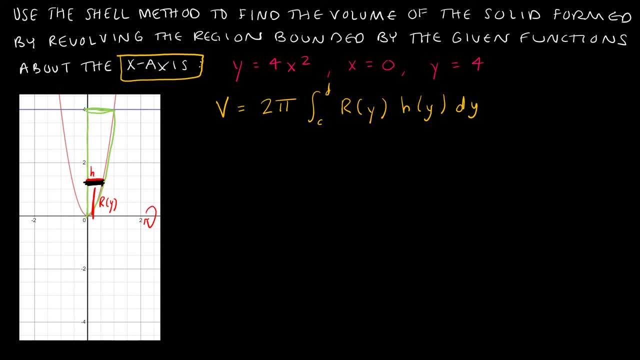 the distance across. So that's our height. So, just as I did before, I want to think about what each of those values would be. So what would be my radius? Well, my radius is just going to be the y value. So whatever value I have for y, 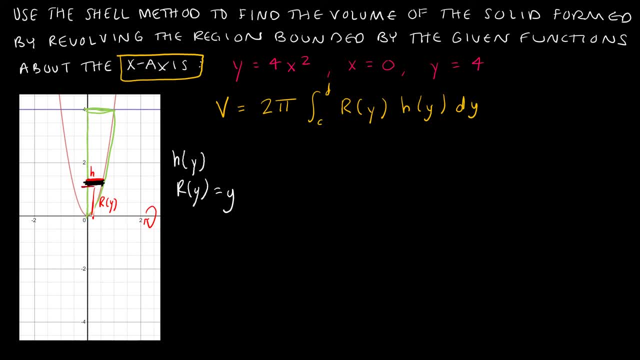 is going to be equal to my radius of my figure. The h of y is kind of like the r of y in our last example where I had to do a little bit of work. So the r of y is going to be whatever my x value is. 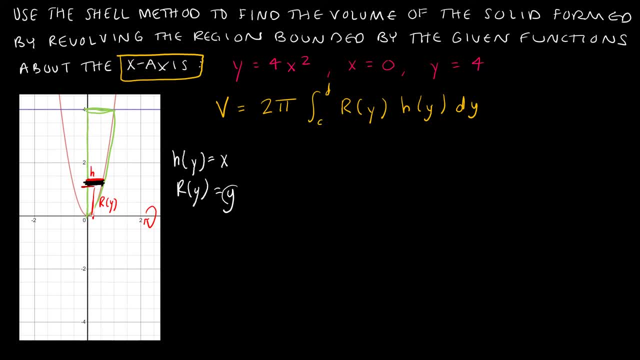 because it wasn't our last example. But in my last example I had to do some work to get the value in terms of x. So that's what I'm going to have to do now is get some, do some work to get this. 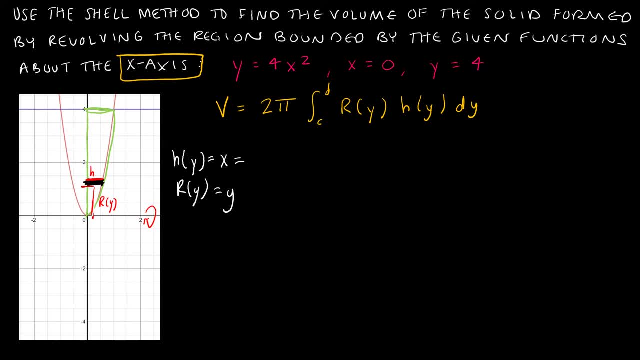 value in terms of y. So again, I'm going to use this function because that function would represent the value. But notice that function is in terms of y, So y equals, so it's in terms of x. excuse me, I have y equals 4x squared. I need to isolate. 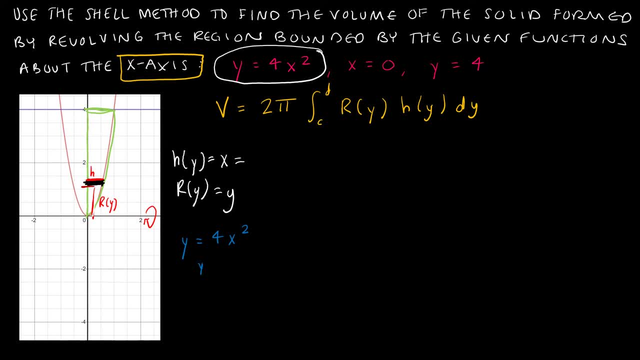 the x. So I'm going to take y divided by 4 to be x squared. Taking the square root plus or minus the square root of y over 4 gives me x. Now, keep in mind, I just want the positive. 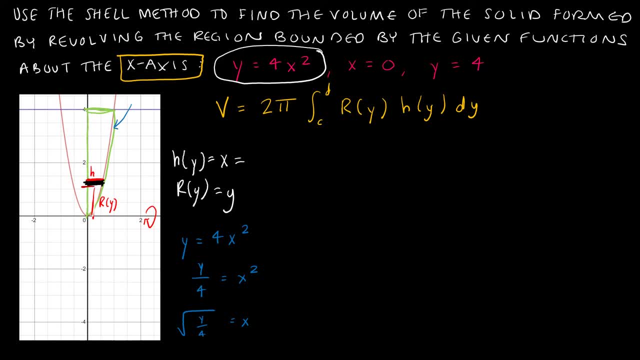 side. So I only need the positive. I don't need plus or minus, And I would take the square root of y over the square root of 4.. So I'm just going to simplify that: to the square root of y. 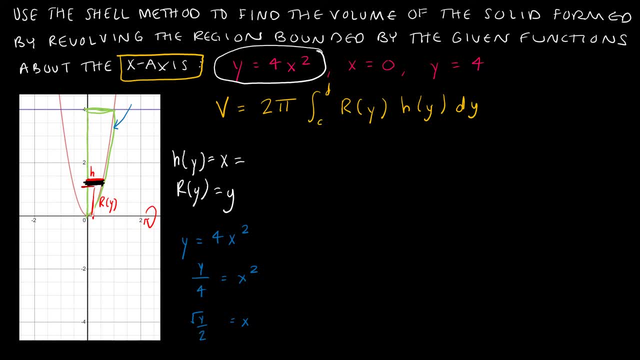 over 2.. Because the square root of 4 is 2.. So that is now going to be radical. y over 2 is going to be my height, because it is my function written in terms of y. So now let's find our solution. I have 2 pi. 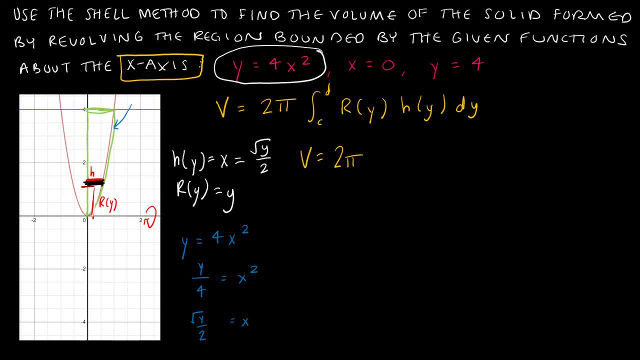 And then again I need to know what are my limits of integration. And looking at this, I can see that I'm using the y values And I'm given the limits, so I don't have to do any work. So from 0 to 4.. 0 to 4.. Again, the radius we said was y. 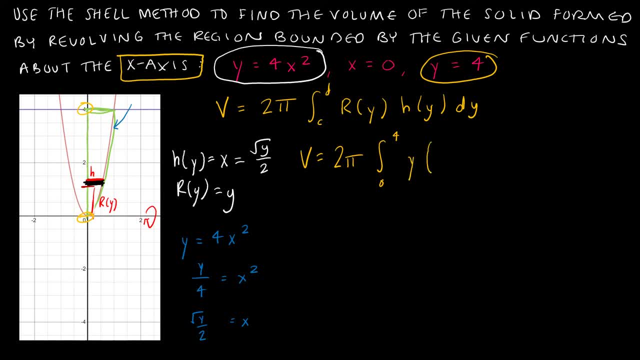 h of y is the height, which is radical: y over 2.. And dy. Now I'm going to try to do just a little bit of simplification. I'm going to take this 2, which is essentially like a 1 half because it's divided by 2. And I'm going to move it to the 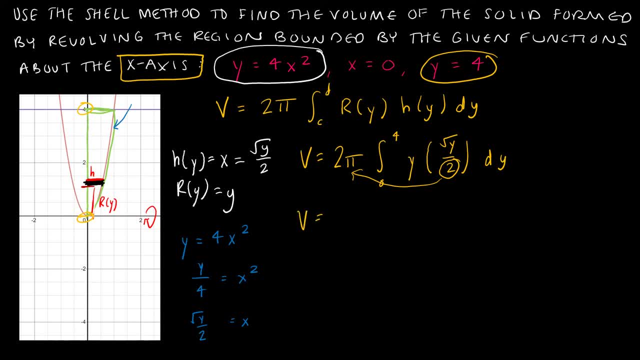 outside. So I have 2 pi And then I have divided by 2. So on the outside now I just have pi And then again from 0 to 4. And I want to combine now this y and this y, So I have y to the first And then I have y to the 1 half, just as I did before. 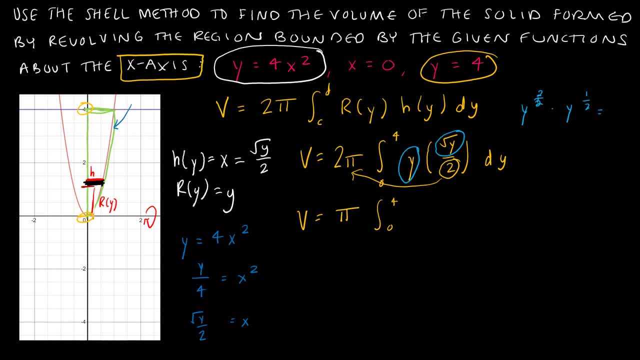 Which gives me y to the 2 halves, And then y to the 1 half means I can add to get y to the 3 halves. So that's what I have here: y to the three-halves dy, and then I'm going to integrate. So I have pi on the outside. 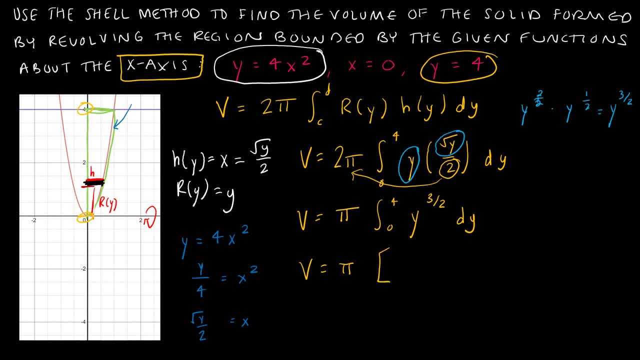 Now I have y to the remember. I'm increasing that exponent by one, so it's y to the five-halves and I'm dividing by five-halves. but instead of dividing by five-halves, I'm going to multiply by. 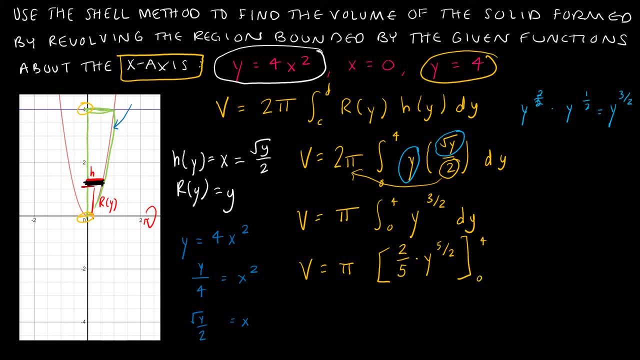 two-fifths again from zero to four. So it's okay for me to take this two-fifths out to make things a little simpler. So I have two-fifths pi and then I'm going to use y to the five-halves with 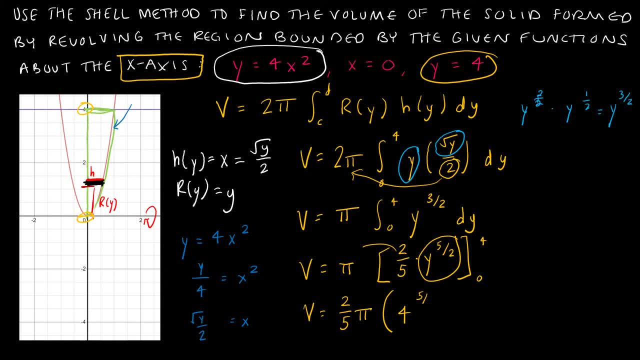 four and with zero. So this is four to the five-halves minus zero to the five-halves. We know that zero to the five-halves is just zero. so four to the five-halves, just as we had it. 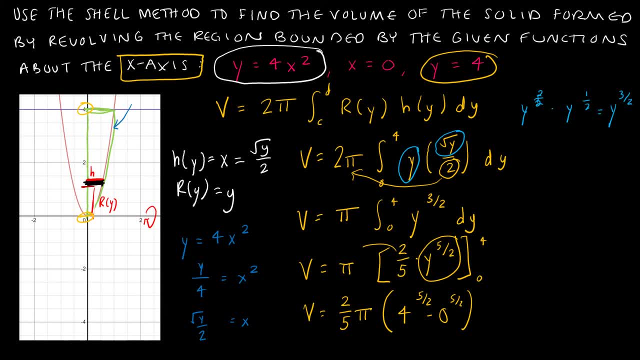 before means to take the square root, kind of running out of room here. but remember, four to the five-halves is the same as four to the one-half, to the fifth, and four to the one-half just means what's the square root of four. 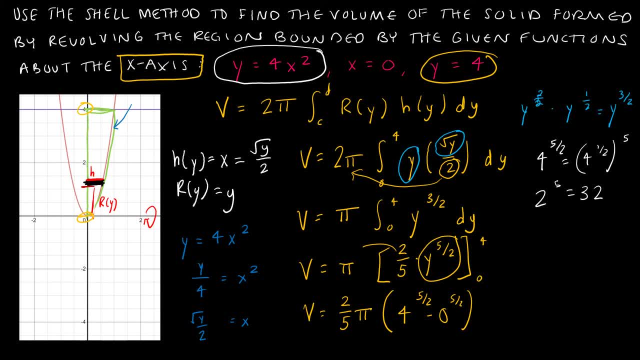 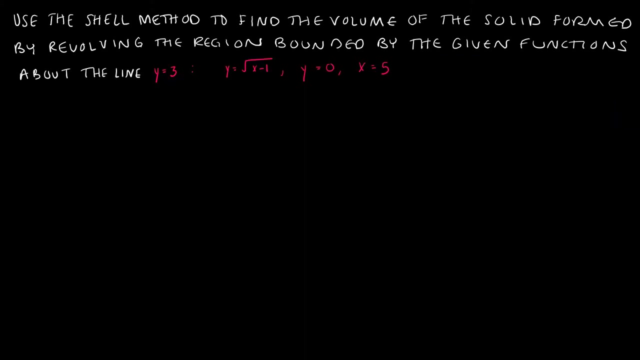 so that's two to the fifth, which is 32.. So down here I have two-fifths pi times 32, which is 64, 64 pi over five cubic units. Let's do one more example together, and frankly I'm just throwing everything at you in this example. 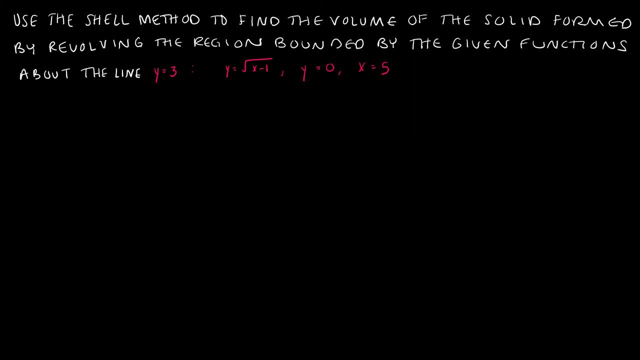 So this one's going to take us a little bit and it's going to be kind of a tougher example, but let's go through it together and hopefully we'll get through okay. So we're going to use the shell method to find the volume of the solid formed by revolving the region. 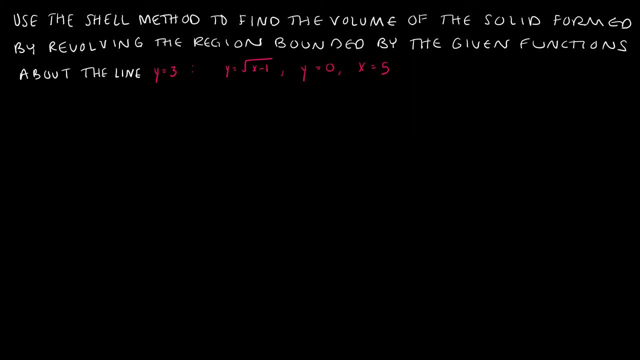 bounded by the function, y equals the square root of x minus one, y equals zero and x equals five about the line y equals three. So this is our solution and we're going to use the shell method to find the volume of the solid. 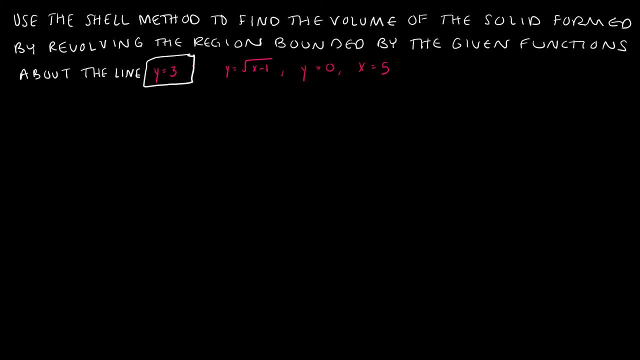 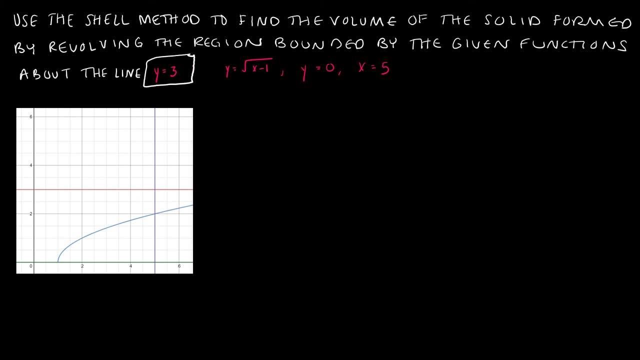 and this is our first time of revolving around anything other than one of the axes. So, again, I went ahead and graphed this, just so we could get an idea of what the region looked like. We're looking at this region bound by: y equals zero, x equals five and my function: y equals radical x minus one. 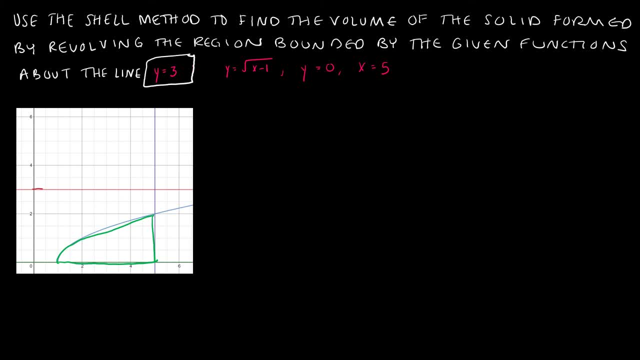 and we're revolving around a different line. now We're revolving around this line, which is y equals three. So again, if I were to revolve around this line, I would be revolving around this line, which is y equals three. So again, if I were to revolve that, it would look. and I'm not a very good artist, as we've already talked about. 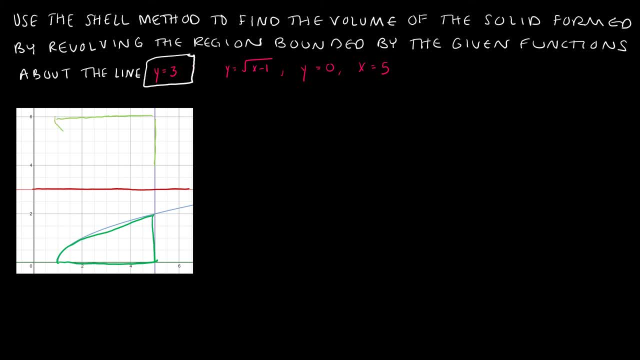 it would look something like this. You get the basic idea Again. what am I going to do? I'm going to draw the line that is parallel to the axis of revolution, and this is where it gets a little bit tricky, because, up to this point, 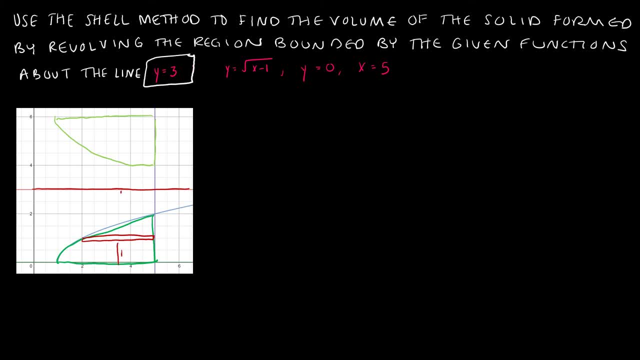 I've always had this value being r, which was just the same as the y value. Now I need this value to be r, So how am I going to fix that? Well, I know that, as we just said, this value is y. 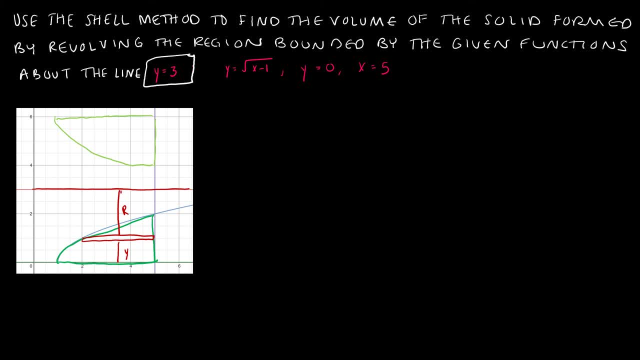 So from the x-axis to our function is the same as the y value And I need the opposite of that, So I need the other side of that line. Well, what's the total length of this line? The total length is three because obviously y equals three. 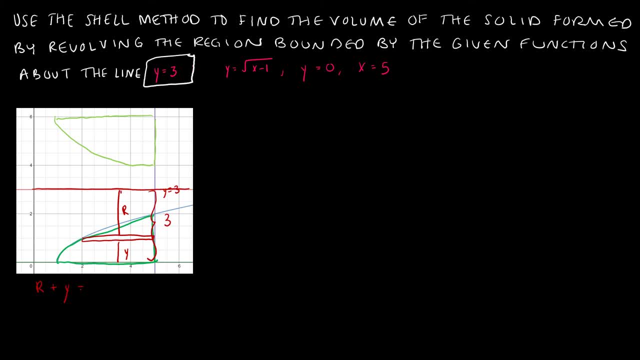 So if I know that together, r plus y has to equal three, then I can find that r is equal to three minus y. So that's the function I'm going to use for r, And, good for us, it's already in terms of y, so I don't need to do any additional work. 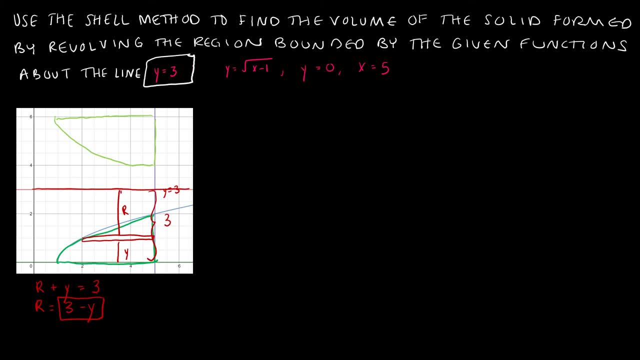 Now, if I were to draw a line that is parallel to the axis of revolution? Now, let's use that same thought process to find h, Because, again, just as a reminder, I'm looking for two pi. and then this is: from c to d, of r, of y, h, of y dy. 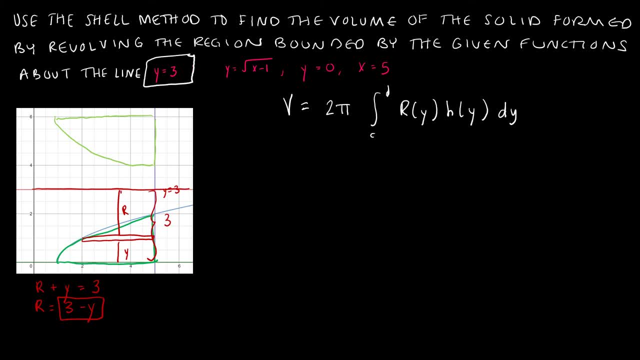 So I've just found r of y, Now I need to find h of y, So let me switch colors here. So now I'm looking at: what is this? This distance, That's what I want to find. Well, I know that from here to here is x. 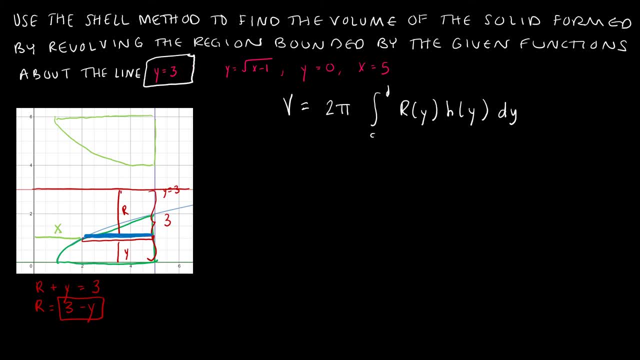 That's the x value, just like the other value was always y. So same idea. So if that value is x and this value is h, which I'm trying to find, I can use the same concept I did before and say: total, this is five. 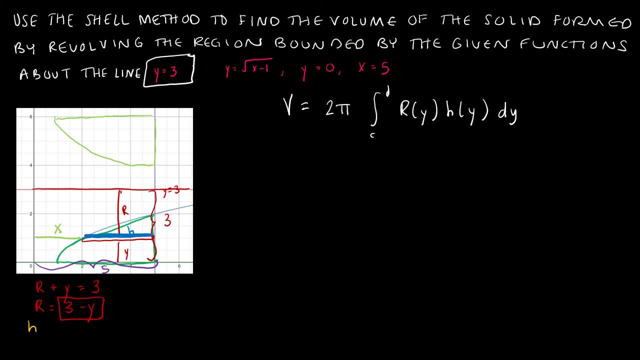 So that means that h plus x is equal to five. So h is equal to five minus x. Now, the problem with this one is that this is written in terms of x, and that's not okay, because I'm integrating with respect to y. 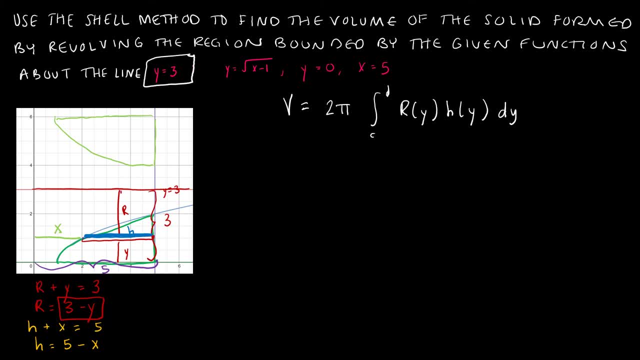 So now I have to do some additional math to figure out how to turn this into with respect to y. So, just as I did before, I'm going to go back to my functions. Remember, I know that y is equal to root x minus one. 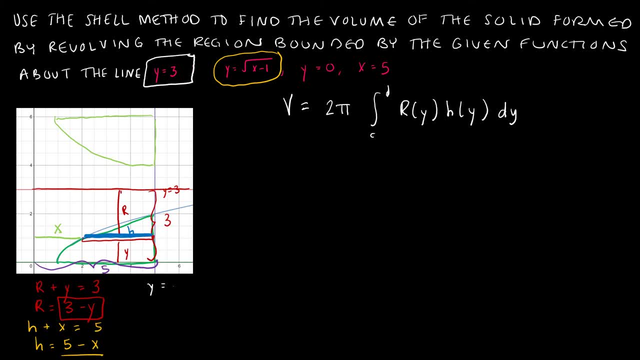 So let's do some math here. If y is equal to root x minus one, I can square each side. to get y squared equals x minus one, And again I'm trying to get x by itself. So I'm going to add one to each side. 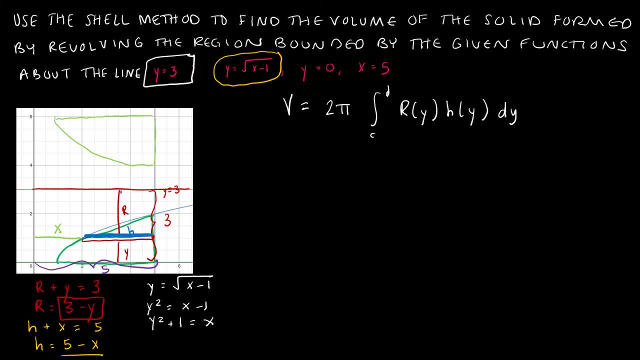 So I get: y squared plus one is equal to x. So I'm going to write this as: five minus y squared plus one, which reduces to again: five minus one is four. So four minus y squared. So this is going to be my h of y: four minus y squared. 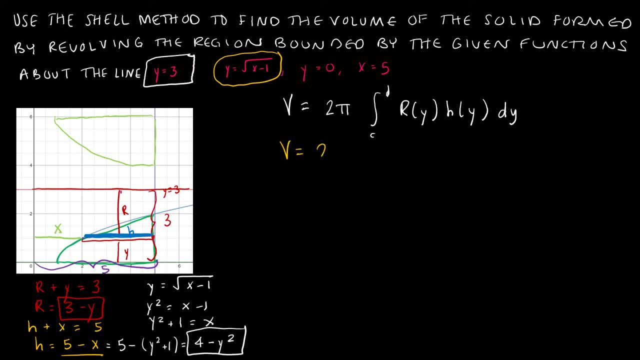 So let's go back up to my integral now and start plugging in values that I know. So we haven't really found the limits of integration, And again, this is with respect to y, Now I know that zero is my lower limit of integration. 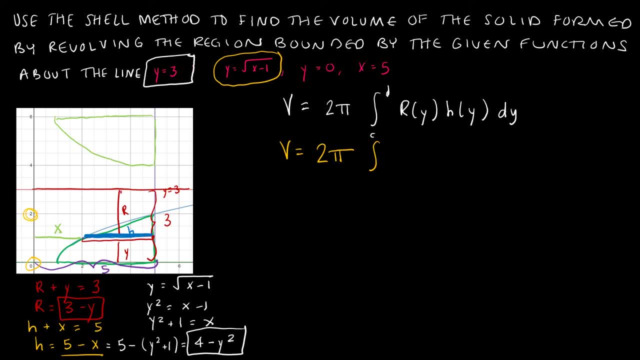 But the question is: what's my upper limit? Now I can look at the graph and cheat a little bit and say, well, obviously it's zero to two, But mathematically, how would I know that it's two? 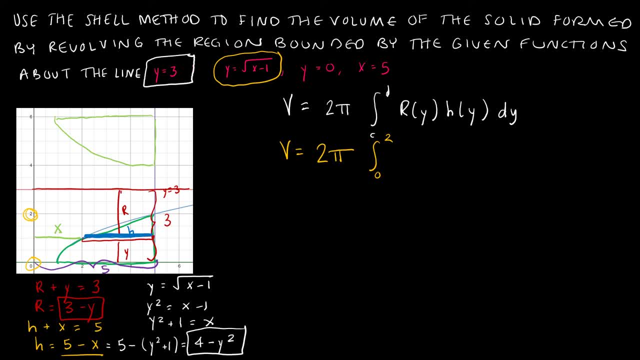 Again, because if I plugged in five, which is this value right here, I could say y is equal to root. five minus one, y is equal to two. So that's going to be this point. right here is five comma two, And that's how I know that two is the furthest that we're going to go on the y-axis. 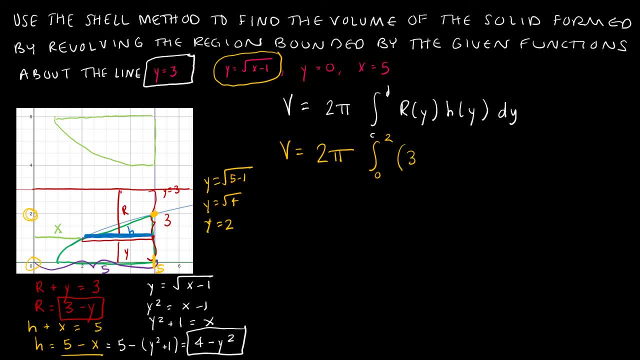 And again. then I'm going to replace r of y with three minus y, I'm going to replace h of y with four minus y, squared, and then dy. So we've done the hard part. Now it just comes down to doing, you know, the algebra. 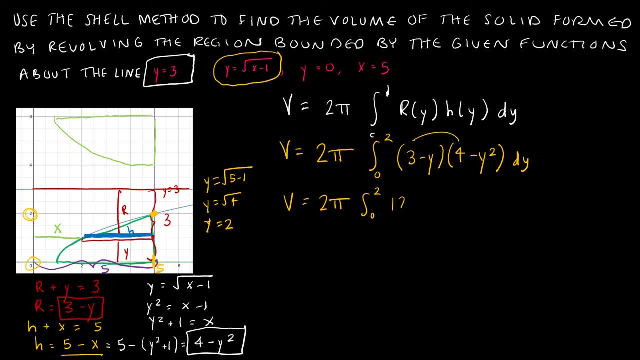 So I'm going to do the algebra, I'm going to FOIL this out, I'm going to get 12 minus three y squared minus four y, and then plus y cubed, And now I'm going to take two pi And then let's go ahead and integrate. 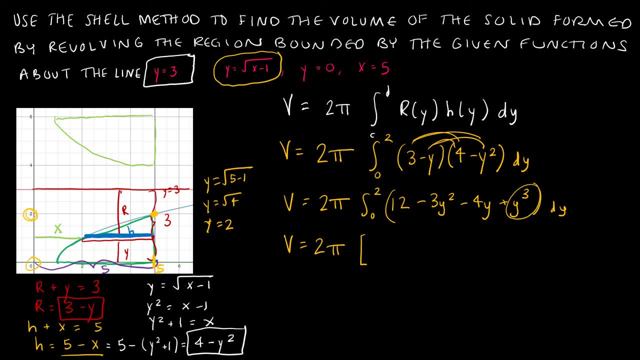 And I'm going to start with this value. So I'm going to go in the normal standard form order. So y cubed is y to the fourth over four And then minus three. y squared would be minus three y cubed over three. 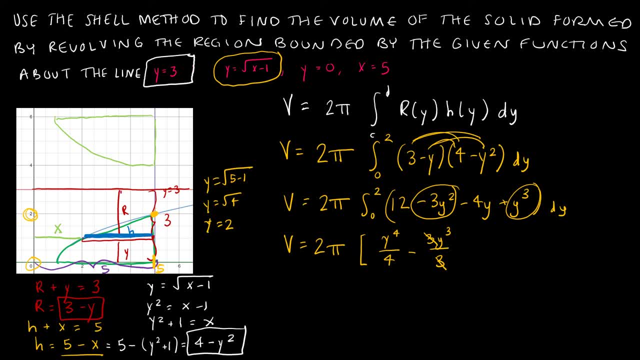 which of course will cancel, And then minus four y becomes minus four y squared over two, which will reduce, and we'll do that in a minute. And then plus 12 gives me plus 12.. 12y from zero to two, So now I have two pi. 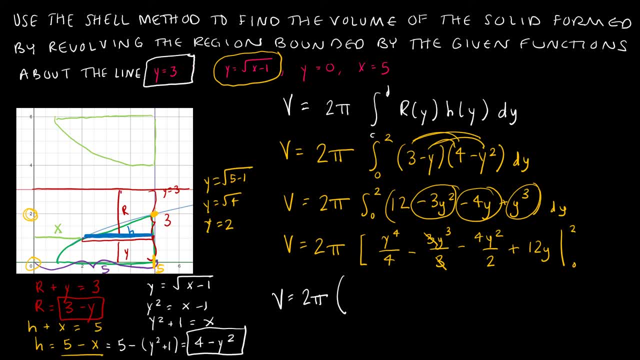 And then y cubed over four again, starting with the two. So two to the fourth is 16. divided by four is four. The three is canceled out, So it's just y cubed. So two to the third is eight. 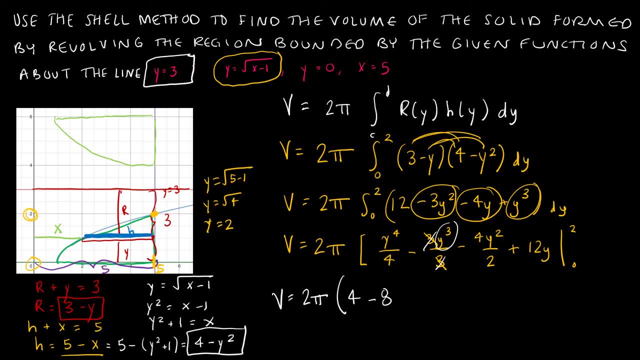 So minus eight, Two squared. Let's go ahead and reduce this: This is two, This is one, So it's just two y squared. So I'm subtracting two times two squared, So that's minus eight And then plus 12y. 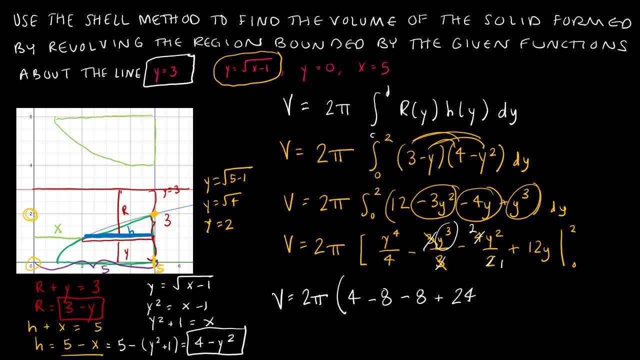 So plus 24.. And then, if you'll notice, if I plug zero in, I'm just going to get a lot of zeros. So it's just minus zero. So now I have two pi, And then I have four minus eight, which is negative four. 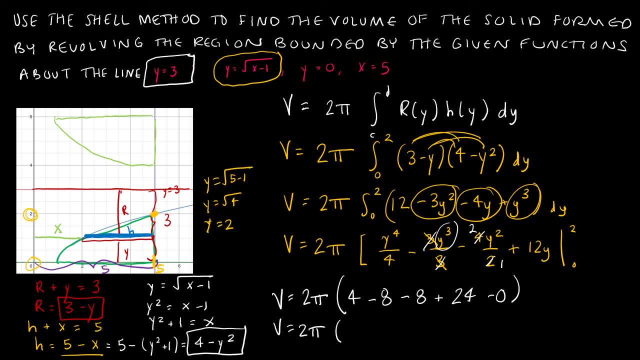 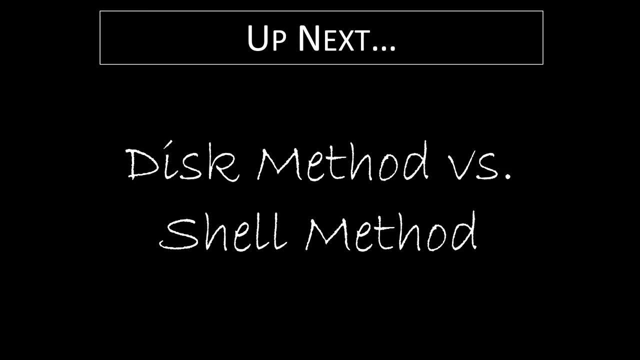 Minus eight, which is negative 12.. Plus 24 makes it positive 12.. So my final answer is 24 pi cubic units. Great job, especially on that last example where I threw quite a bit at you at once Coming up next. we just want to take a look. 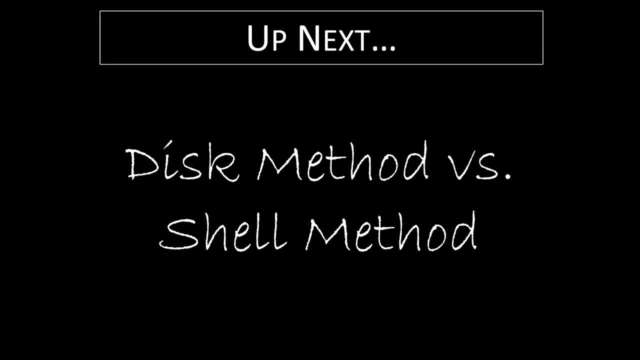 at when is it appropriate to use the disk method and when should we use the shell method?